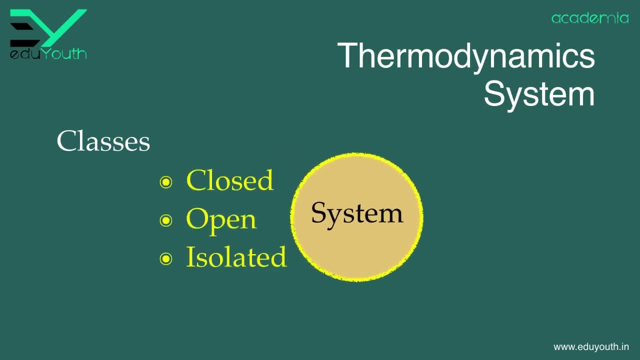 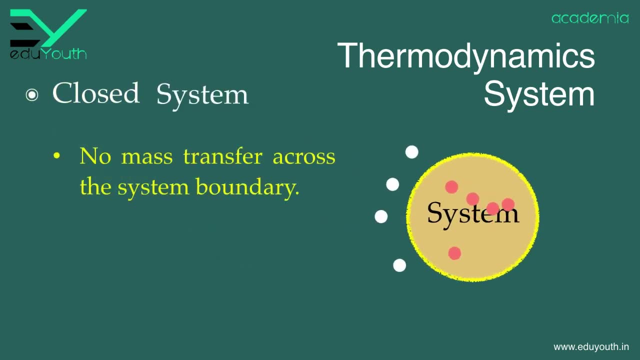 classes of system: closed system, open system and isolated system. the closed system is a system of fixed mass. here there is no mass transfer across the system boundary. neither mass is entering into a system nor coming out from the system. there may be energy transfer into or out of the system for 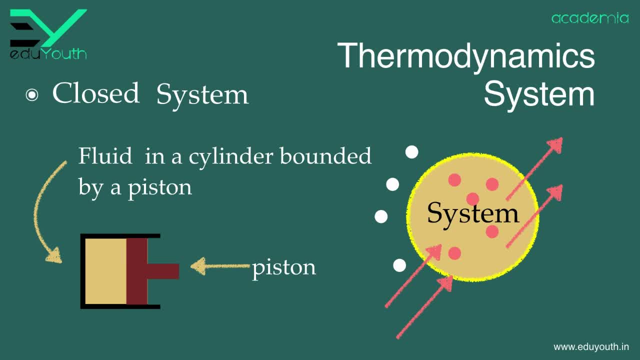 an example: if you take a certain quantity of fluid in a cylinder bounded by a piston, it's constituted a closed system. here, only possibility of interaction is the heat between the system and the surrounding. now the open system is a system in which matter crosses the boundary of the system. 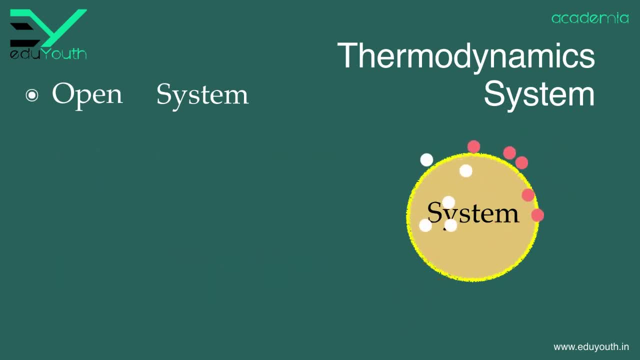 and there may be energy transfer also. for an example, an air compressor in which air enter at low pressure and live at high pressure and there are energy transfer across the system. boundary now, the isolated system is a system in which there is no interaction between the system and the 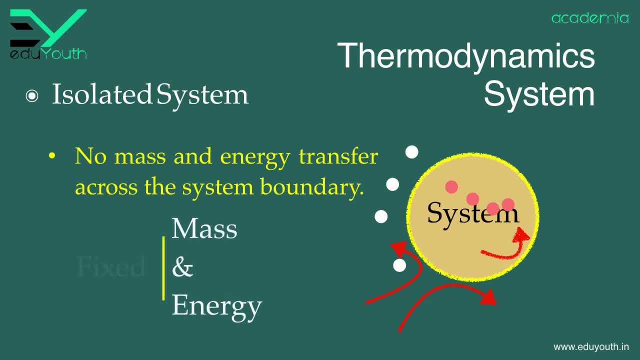 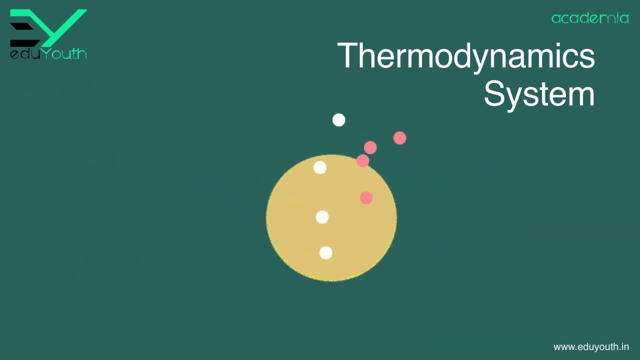 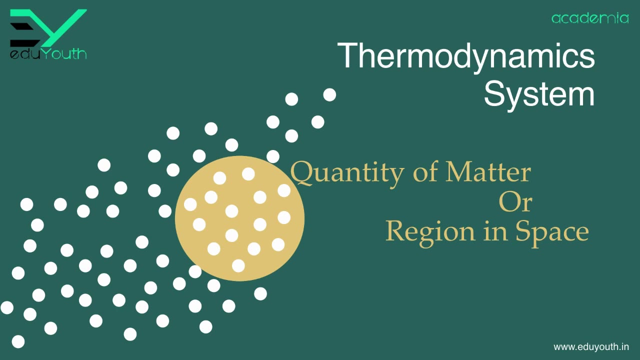 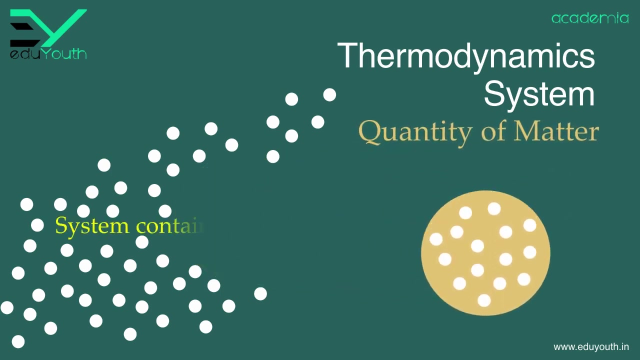 surrounding the mass and the energy is fixed and there is no mass or energy transfer across the system boundary. now, as we know, the thermonix system may be defined as a quantity of matter or resonance space, suppose. if thermodynamic system is defined as quantity of matter, here system contains the same matter, so it's a kind of close system. and if thermodynamic 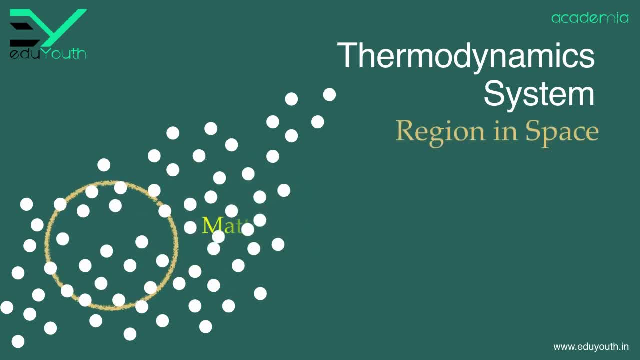 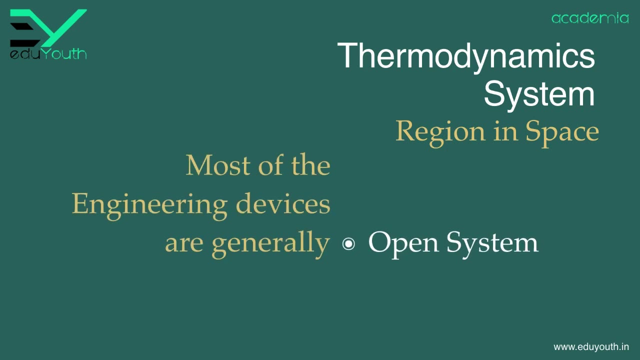 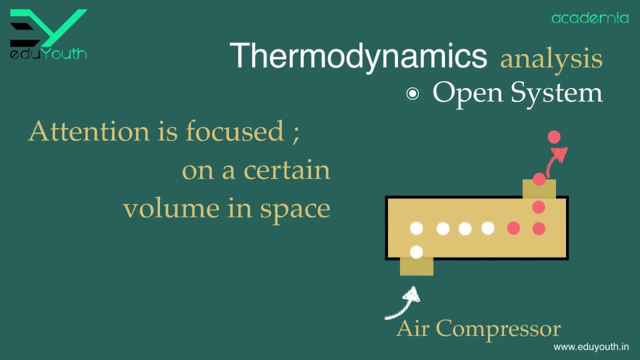 system is defined as reason in space. here matter can cross the system boundary, so it is a kind of open system. We know most of the engineering devices are generally open system. For thermodynamic analysis of an open system such as an air compressor, our attention is focused on a 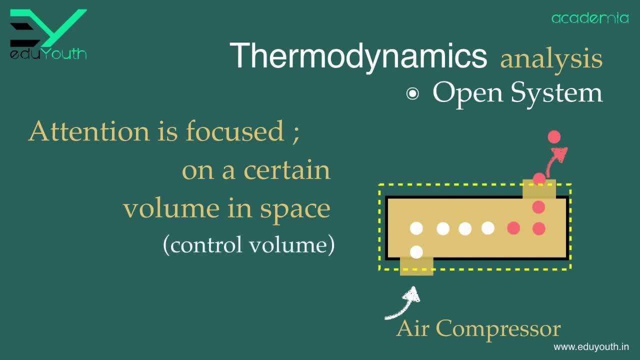 certain volume in space surrounding the compressor, known as the control volume, which is bounded by a surface called the control surface. Here the matter, as well as the energy, crosses the control surface. Also, as we defined, a closed system is a system close to matter flow, though.